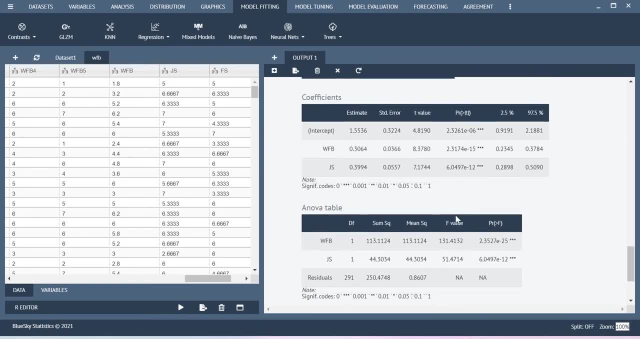 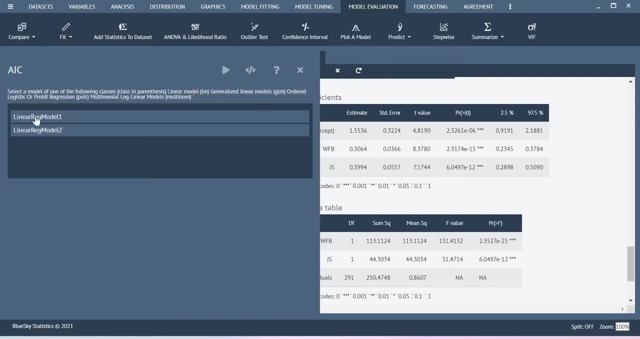 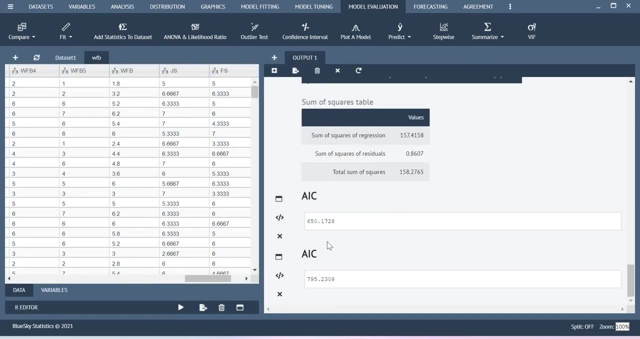 And then execute this. So here I have created another model. Here also, both the coefficients are significant. Now you go to model evaluation, Check the AAC value for regression model 1. And then check the AAC value for regression model 2.. Now, according to this, model 1 is giving better- I mean lower- value than the model 2.. 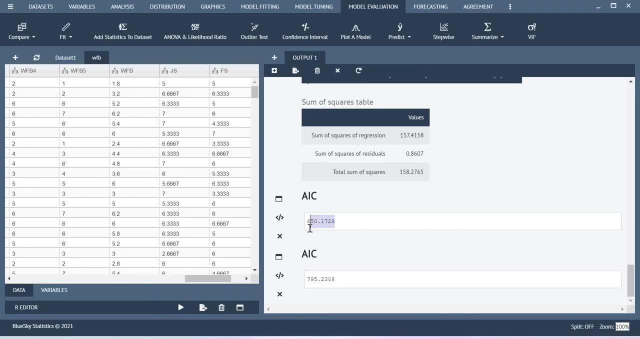 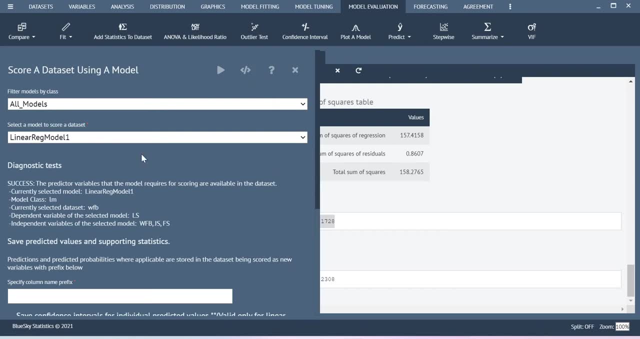 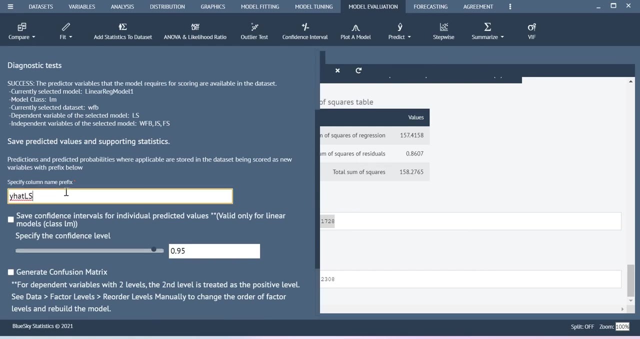 So here I can conclude that model 1 is better than model 2.. Similarly, here you can predict the score for your y. That is nothing but y-head value estimation. So let me consider this as a y-head, Unless you have to give the prefix for this value. I mean computation. 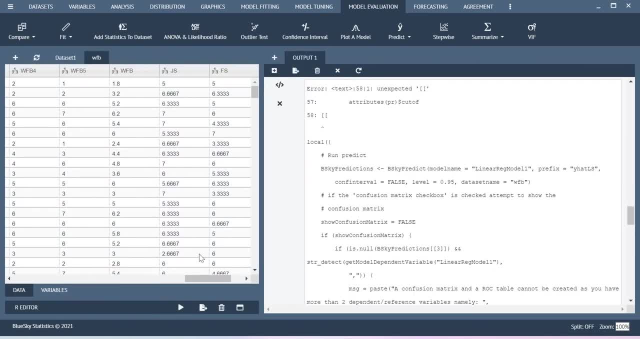 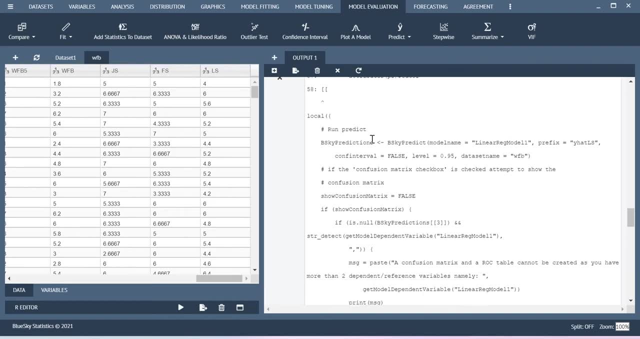 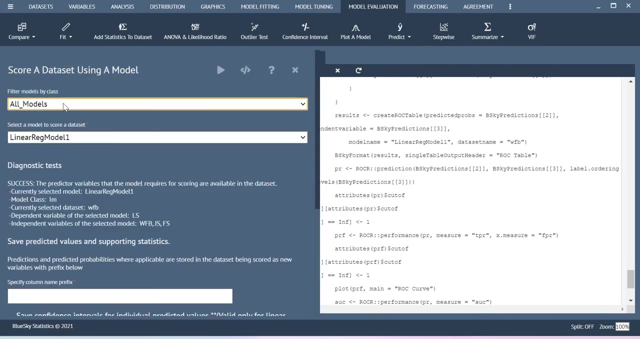 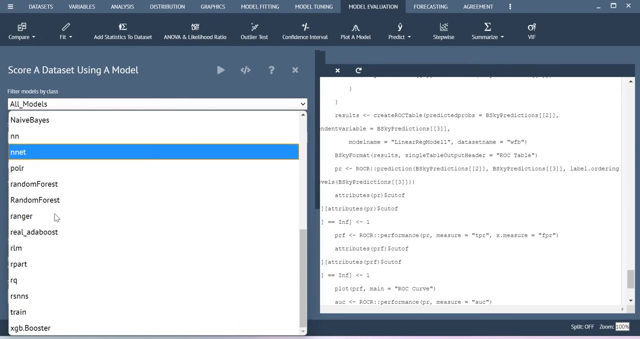 Now you just execute this. If you go back and check your data set, you will be able to get the scores Here. I am getting some error. Let me do it once again. Predict: model scoring. This is for linear regression. I can also select it. 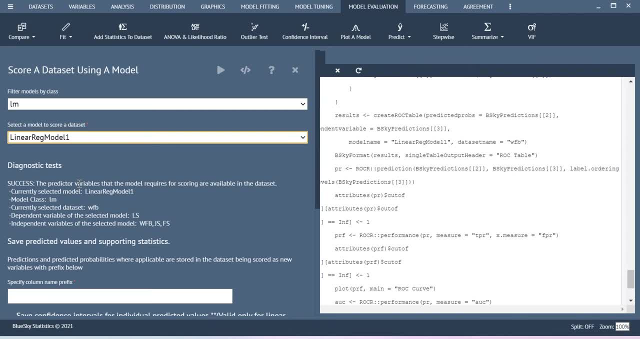 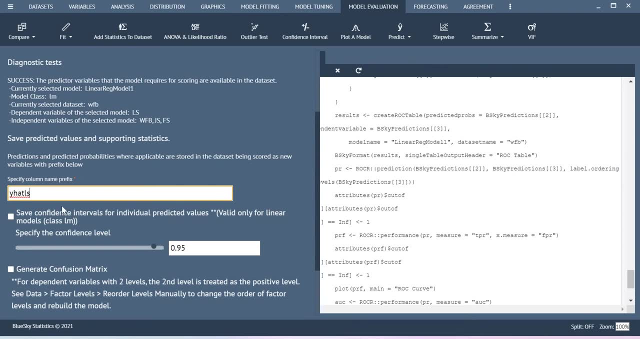 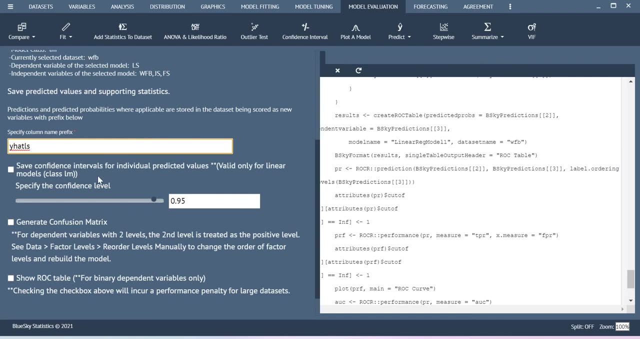 Yeah, lm. This is for regression model 1. Here let me select y-head Ls as a value, prefix value. Now, here, dependent variables are ls. Independent variables are this: 3. Data set is for family balance. That's fine. 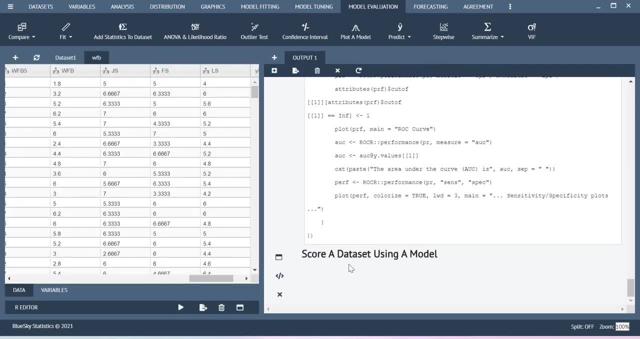 That's okay. Click execute dialog. Yeah, now it is running. If you go back and check your data set here, you will be able to see the output. So, basically, here I have the y-head values. Now, when you want to compute the residual, 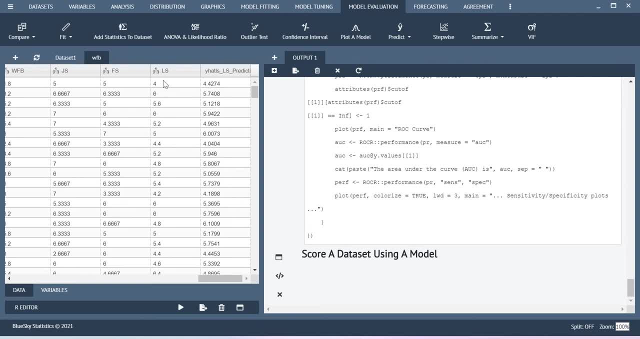 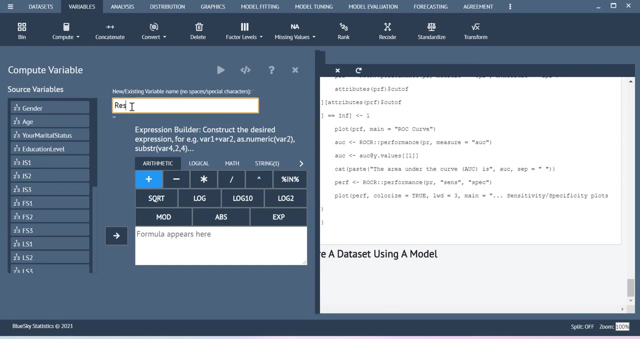 So the residual value is nothing, but you just compare the difference between your observed life satisfaction score versus the estimated life satisfaction score. So in order to do this, you just go to variables, compute, compute. Here the new variable is labeled as residual. 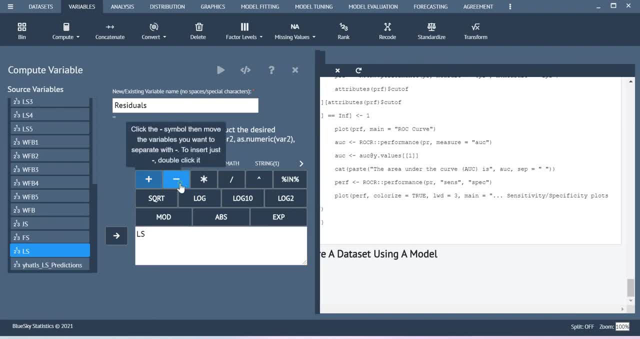 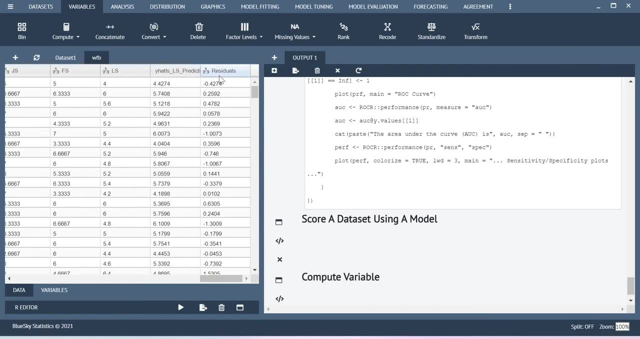 So here you just include: Include the observed score minus estimated score, Execute this dialog, So here you will be able to get the differences in your data set. So this is the way how you can compute the residuals. Similarly, you can also do one more thing. 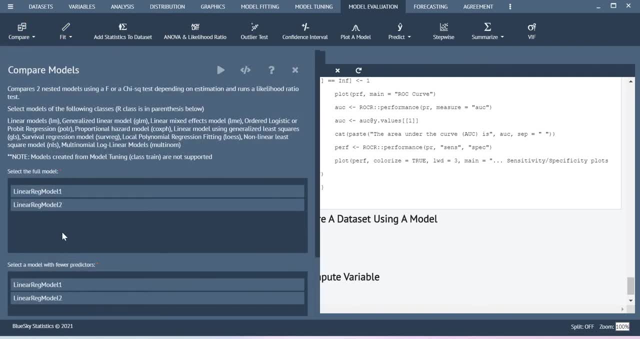 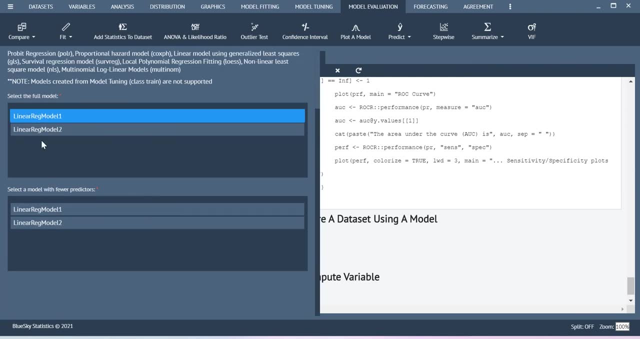 For example, you can compare both the models. Are there any differences, statistical differences, with respect to both the models? that can be done here. in the first, In the first column, you said In the first column, you said In the first column. you said: 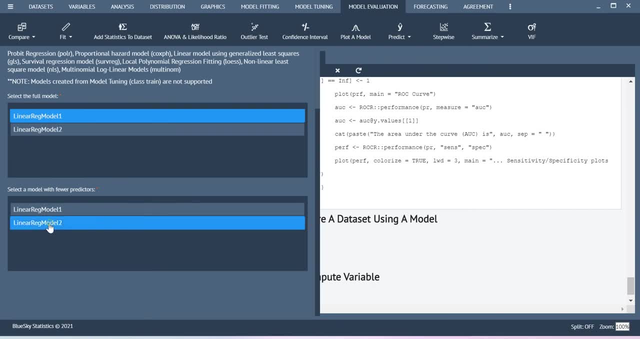 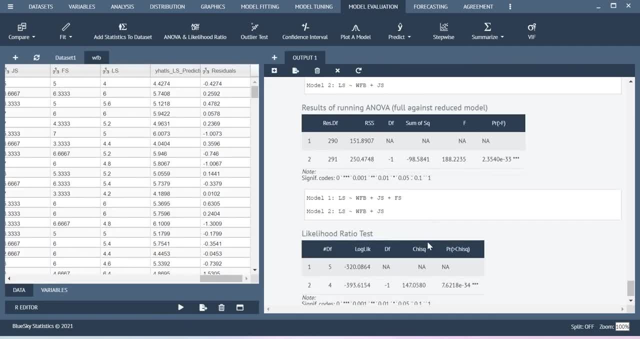 The first column, The first column, The second column, The third column, The fifth column, The sixth column, The seventh column, The eighth column. So here you will be able to get the likelihood function test as well as the on our test. 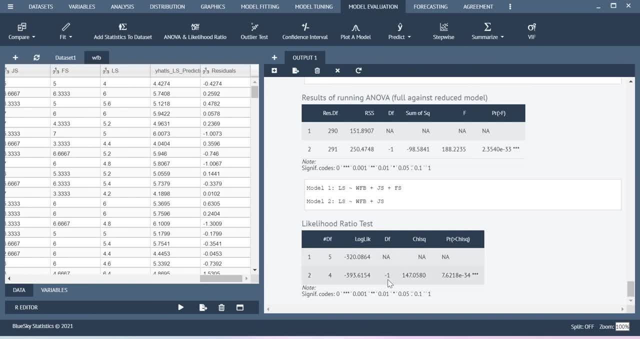 So both the things are seeing that both the models are completely different. I mean, starters are way different. So this is how you can also see them- model differences- using this particular option Here. when you select this plot a model, you will be able to. 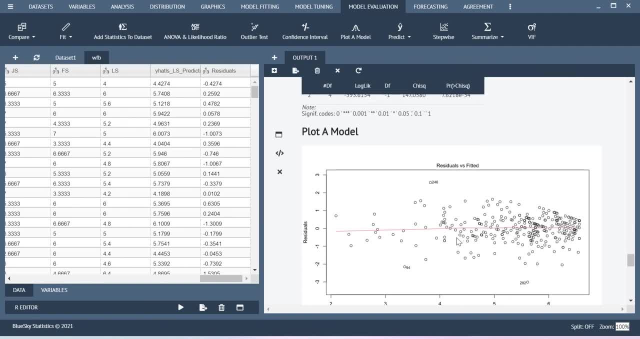 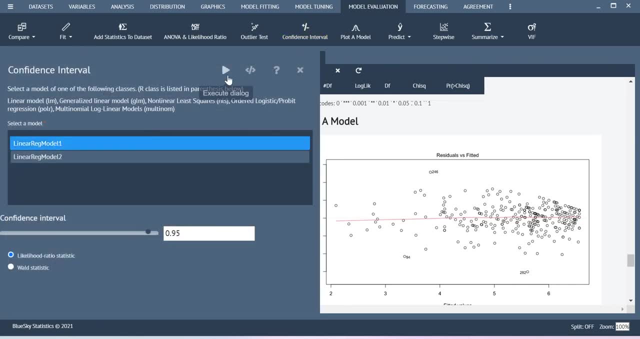 Get some of the plots always Also online pipeline: DWID LEこう yedidaus f, Leonardo Abraham and concepts associated with this regression, like qq plot, and then residual versus fitted and so on. those things can be obtained. similarly, you can obtain the confidence interval for your model coefficients.